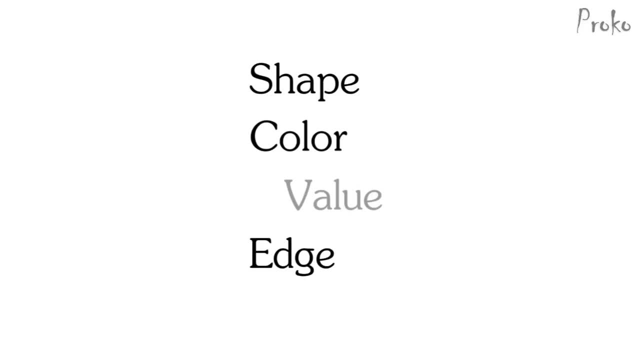 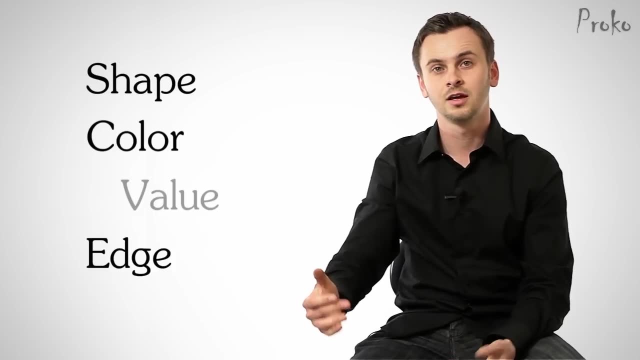 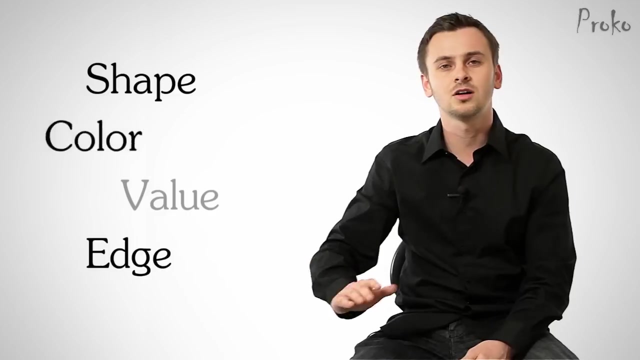 and edge, Because value is just a sub-element of color. It's so important that artists have separated it into its own element, And when we're drawing, it's the only sub-element of color that we can see, And so we forget about the concept. 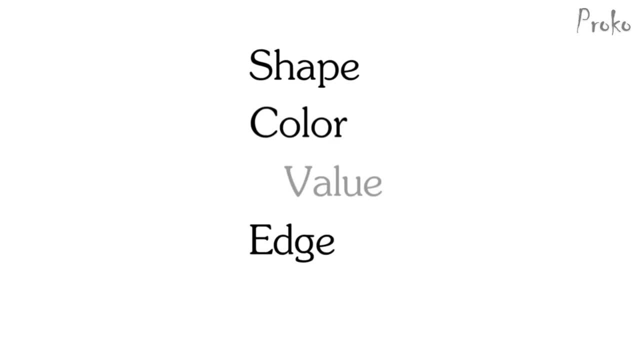 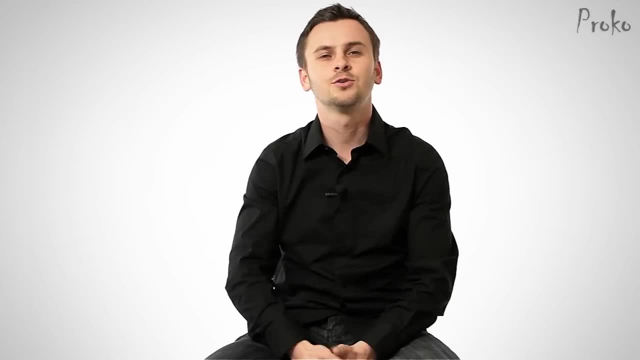 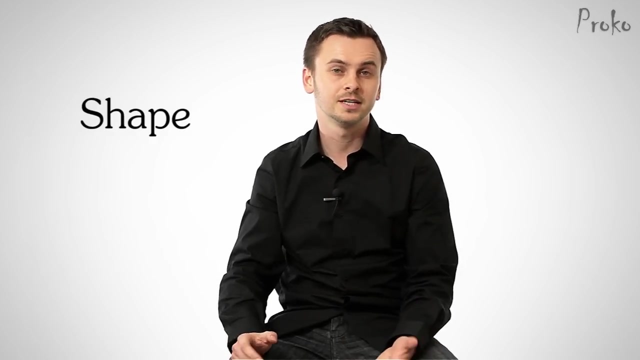 of color for a drawing and we just say value. When we start painting, we introduce the other two sub-elements of color: hue and chroma. So let's go over these elements one by one, starting with shape. Shape is a concept that's familiar to most of us. It's the element that 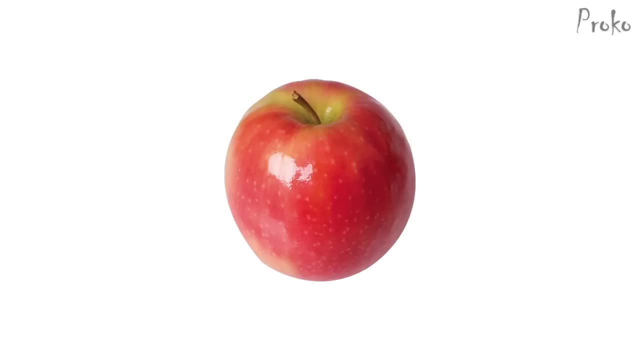 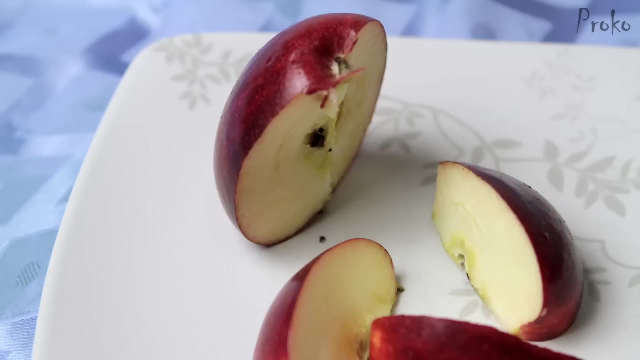 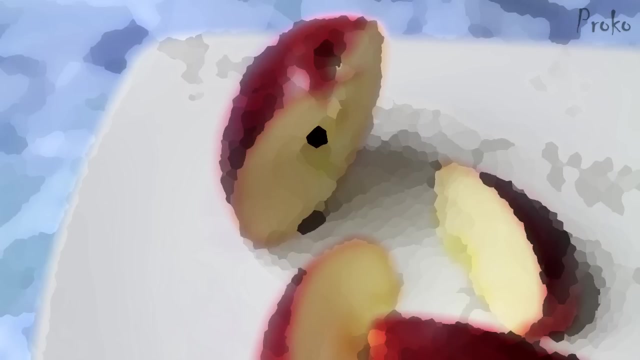 we use to draw as kids. It's the area that something takes up. It's the outline or the contour of all the pieces in the drawing. But it's not limited to just the outline of the big elements. The smaller parts also have specific shapes For the early stages of a. 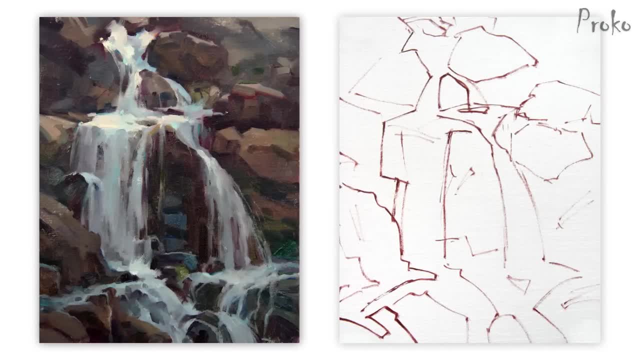 drawing, you want to develop your ability to simplify a shape. This is important so that you can focus on the composition and the breakdown of the big picture. Getting distracted by the big picture is a great way to improve your drawing skills. It's important. 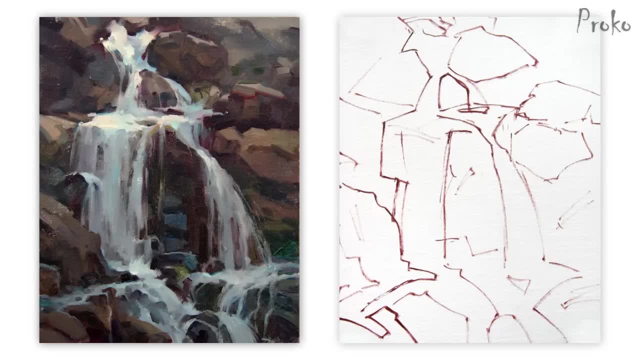 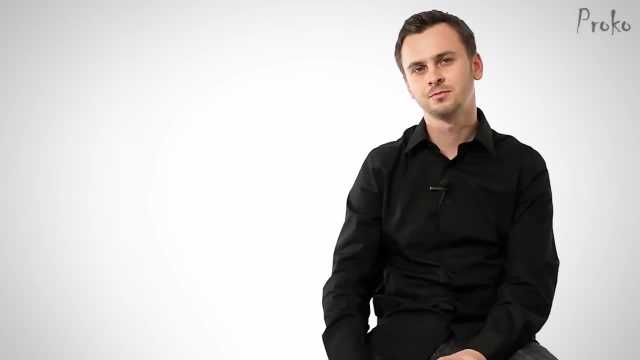 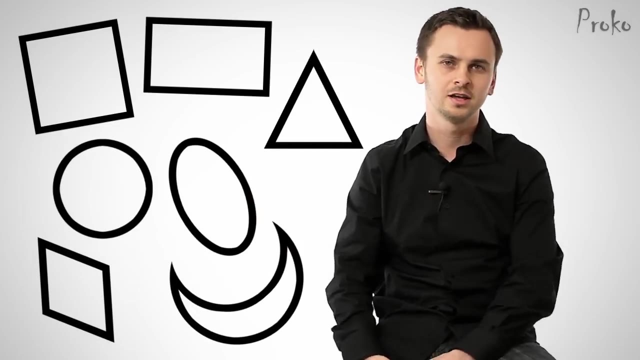 to keep in mind that the smaller details too early can hurt you in the long run. Working big to small is usually a good idea When simplifying. think of geometric shapes: Squares, rectangles, circles, ovals, triangles, diamonds, crescents and so on. These are 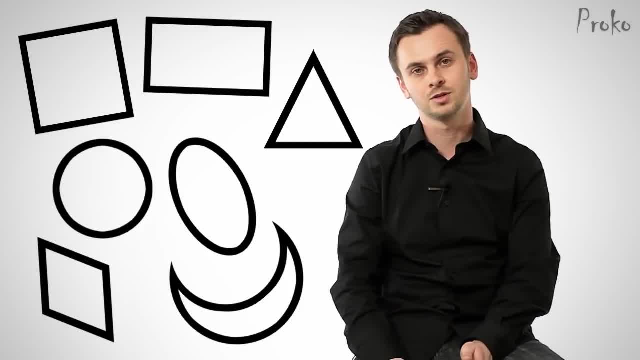 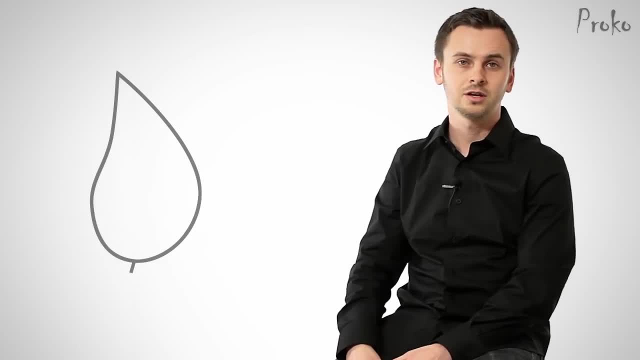 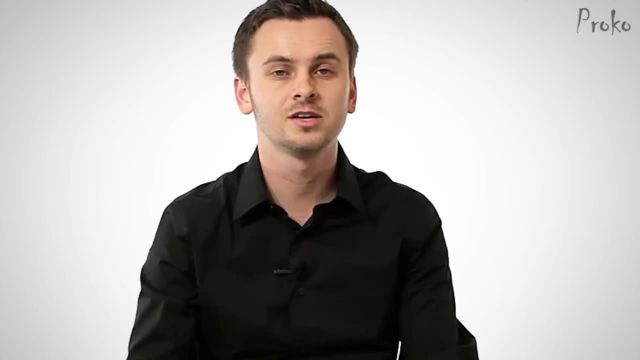 simple geometric shapes as opposed to complex organic ones. For example, this complex shape of a leaf can be simplified in the earlier stages of a drawing And then the details can be found in the later stages. Shape is the most important element to convey the identity of an object. These two shapes 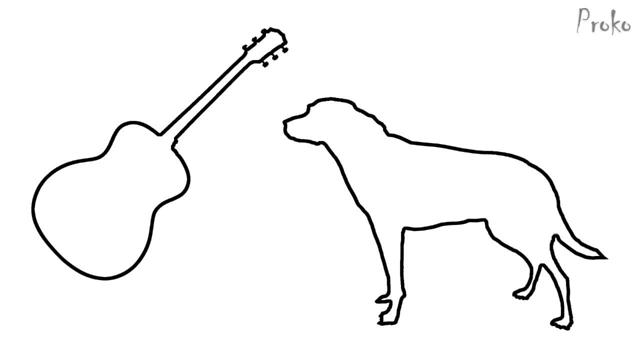 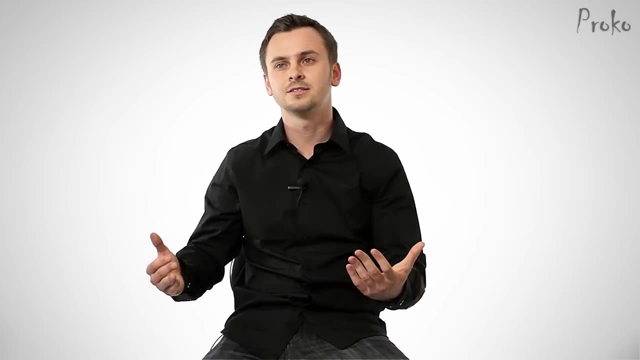 are very different and symbolize two very different things. They are not three-dimensional, but it's still very obvious what they represent just by looking at the shape. That's why shape design is such an important skill to practice and develop. Simply put, shape design is making. 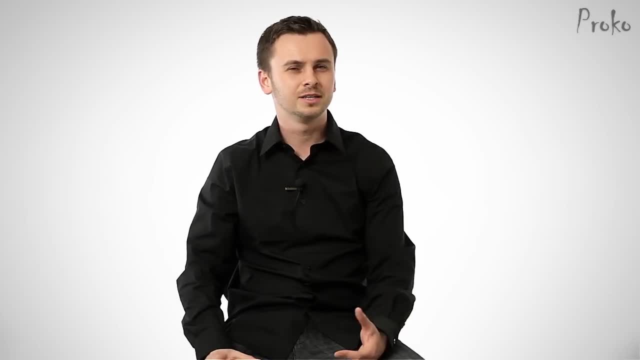 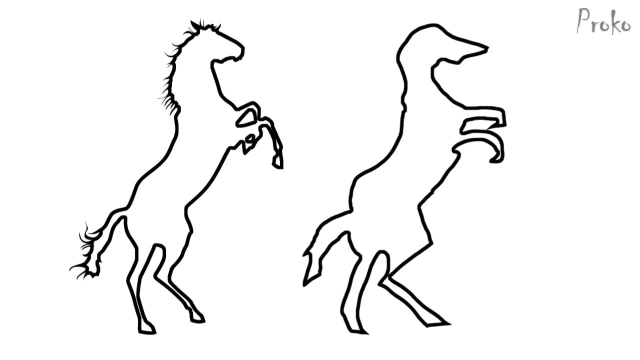 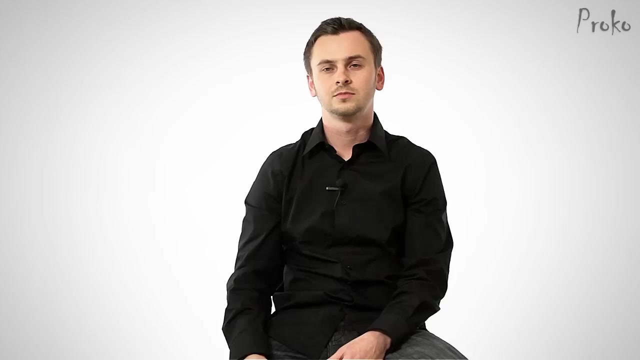 shapes look good. It's a bit arbitrary, but you know it. when you see it, You could say that this shape is better than this one because it's cleaner and more interesting. It does a better job of getting the point across, and doing so in a more interesting way. 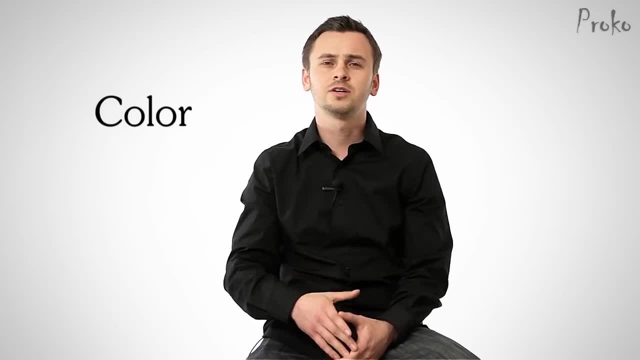 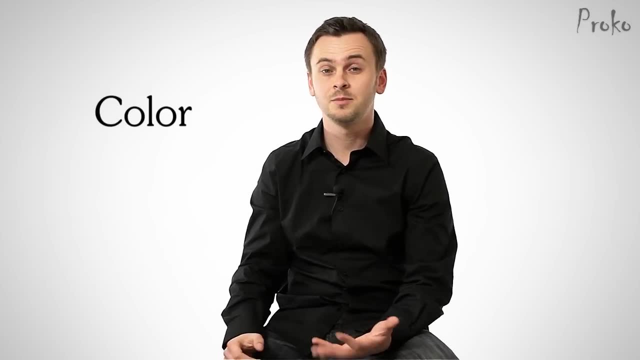 Now let's move on to color. Now I'm going to go into color theory in a bit more depth later, since it's a very complex topic and deserves its own episode and maybe even a whole series of episodes. But right, Right now I'm just going to go over the very, very basics. 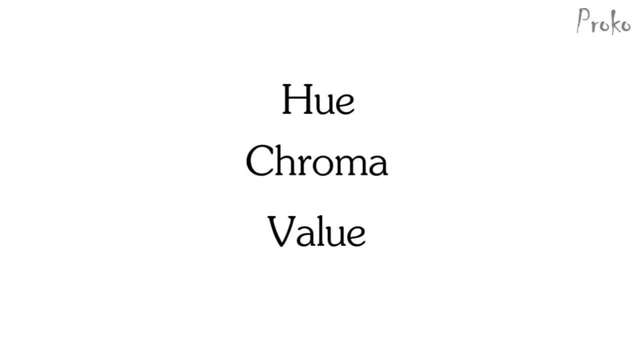 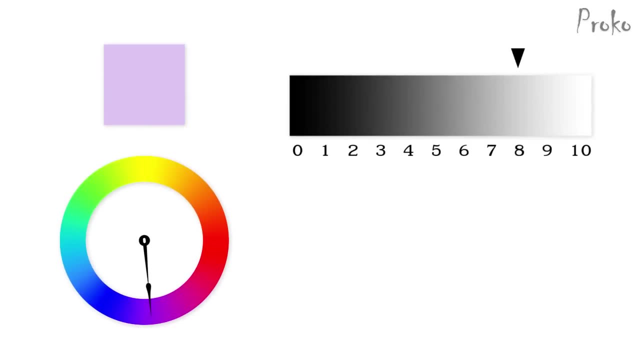 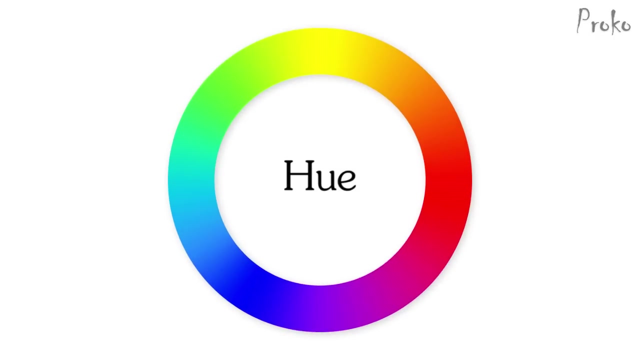 Color has three subcategories: the hue, the chroma and the value. For example, this color has a purple hue, the number 8 value and a medium chroma. Hue is what we typically refer to when we say color: yellow, orange, red, blue, green. 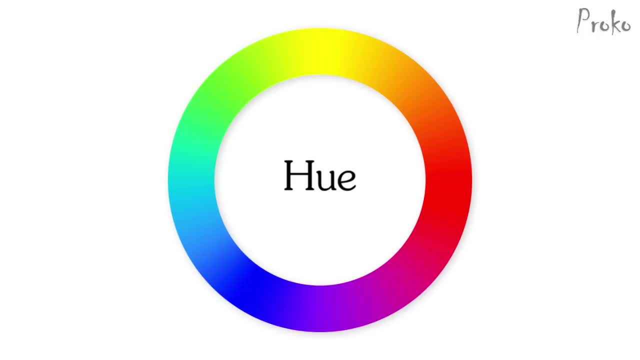 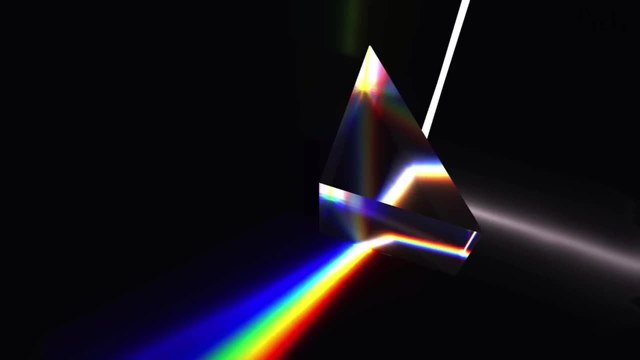 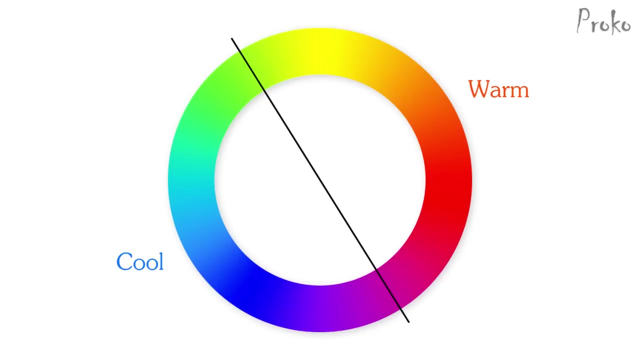 these are all hues. Your traditional color wheel is an arrangement of hues. If you shine a light through a prism, it will break up the light and reveal the color spectrum: The same colors as the rainbow and the same colors as the color wheel. 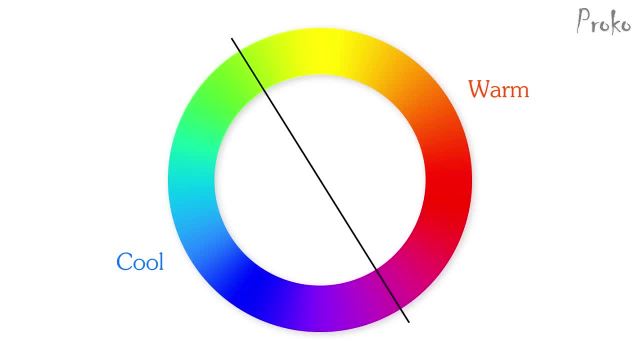 The terms warm and cool are used to describe the two sides of the color wheel. if you cut it in half, The warm family shares orange as a common color and the cool family shares blue as a common color. Think of fire being warm and ice being cool. 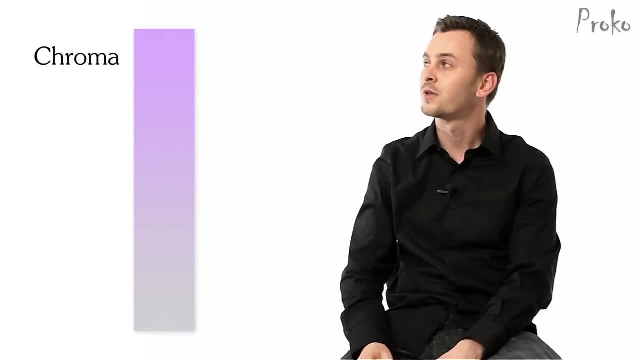 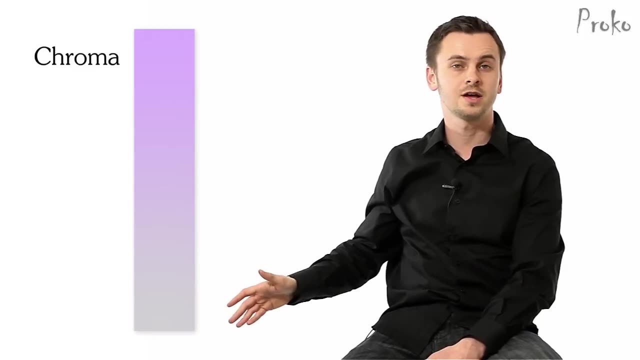 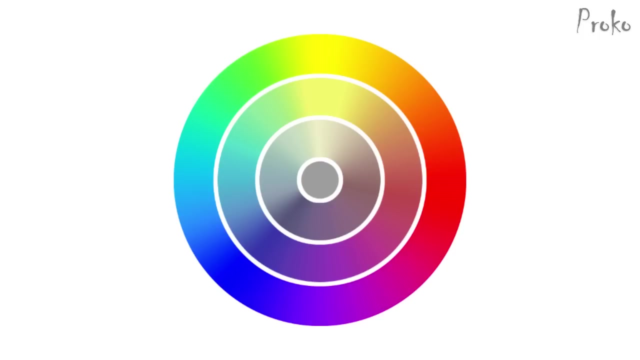 Chroma refers to how pure or how gray the color is. On one end you have the high chroma colors that you see in the rainbow and on the other end you have the low chroma grays with a gradual transition. In some color wheels you'll have the high chroma colors on the outside with a gradation. 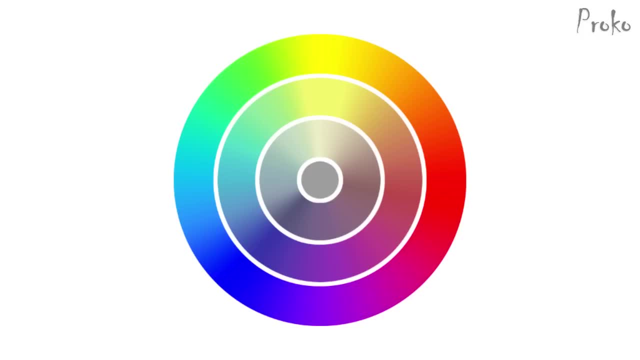 towards gray in the center. You'll often hear people using the term neutralizing a color. This just means lowering the chroma and bringing it closer to gray. There's two ways you can do that. The first is just adding gray to it. 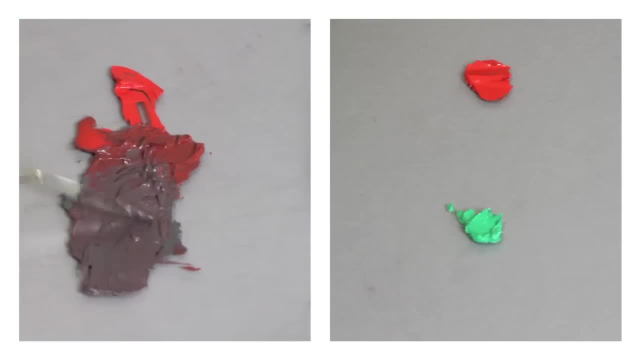 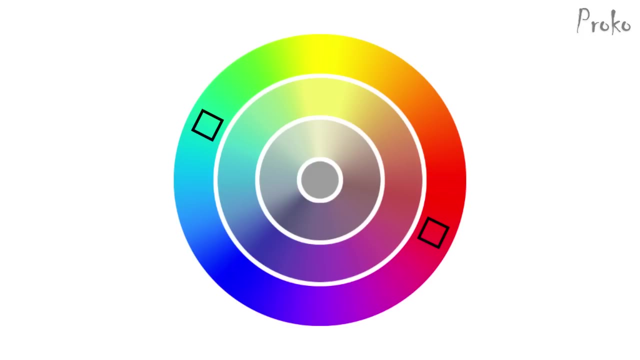 As you'd expect, this will bring it closer to gray. The other way is to add its complement or the color across from it on the color wheel. Mixing these two colors will result in a color between them. Half and half will theoretically make gray. 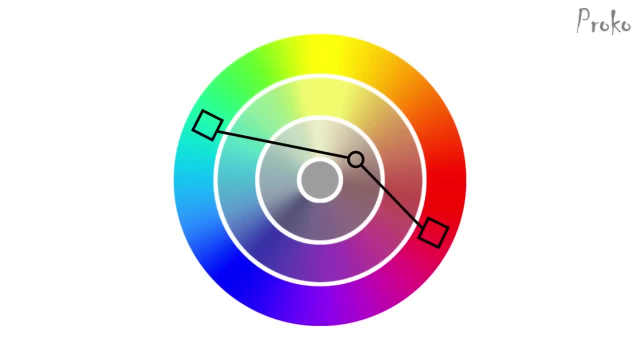 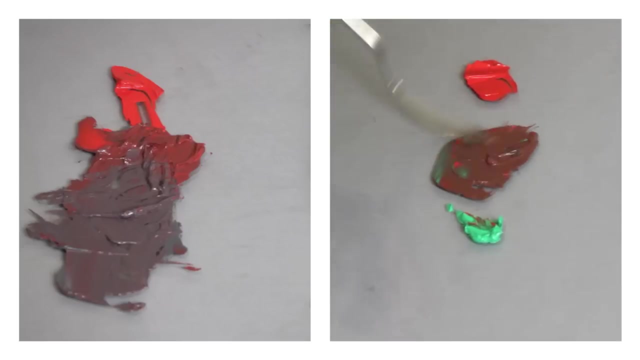 Now, pigment isn't perfect, so you usually don't get that exact perfect gray, But you'll definitely bring it closer to gray Depending on the ratio. you mix will result in a color somewhere in between the two. So if I just add a little bit of green to the red, I'll still have a red, just a lower. 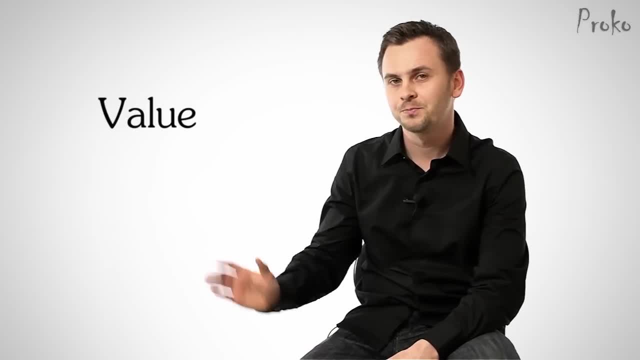 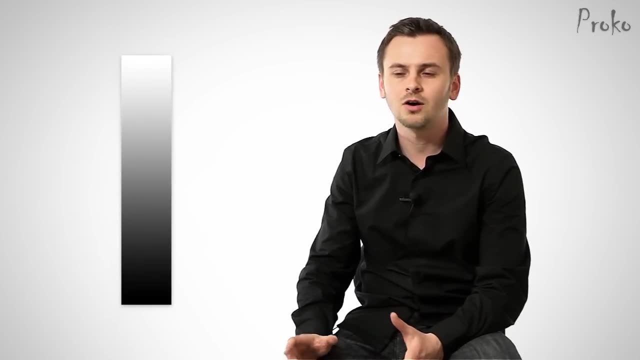 chroma version. Okay, let's move on to value. Value is how light or dark a color is. There is an infinite amount of values, But artists like to say that it's just a color. They like to simplify it to a finite scale, 0 to 10.. 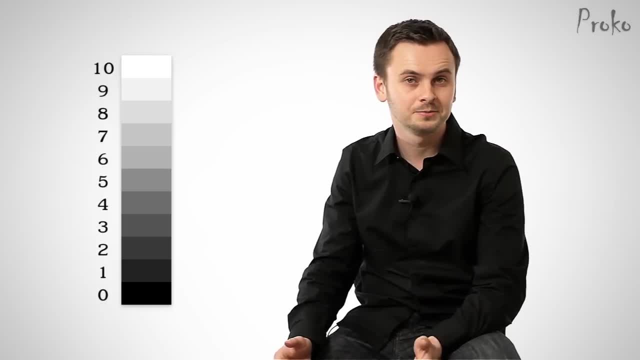 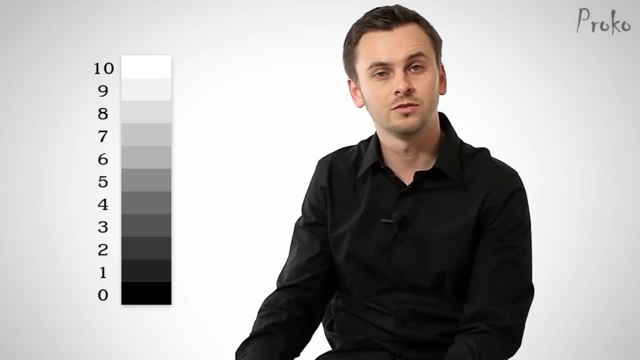 It's a lot more manageable that way and easier to communicate. A teacher might say: make that shape one value darker And you'll know roughly about how much one value is. Drawing with charcoal we don't see color, since everything is grayscale. 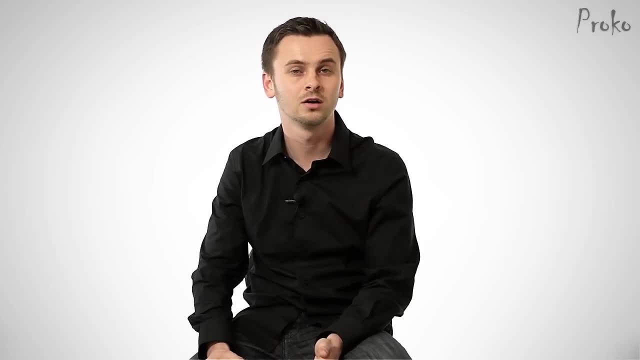 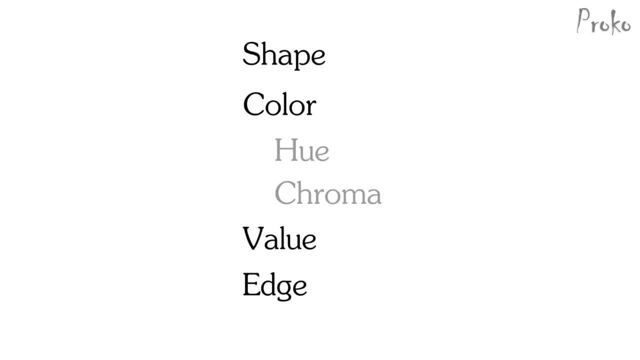 Or a better way to put it is: we don't use hue or chroma. The only part of color that we see is value. So many artists have separated value as its own element and say it's more important than the other elements of color. 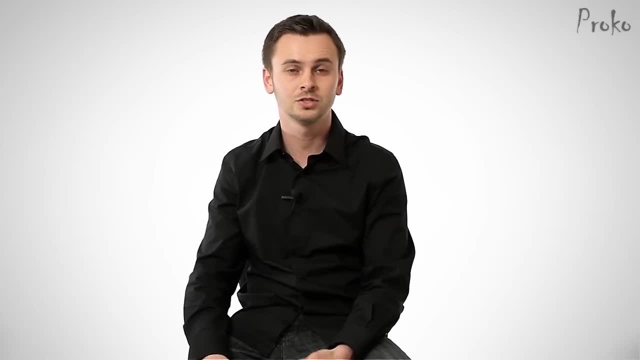 You can have a very beautiful drawing without using color, Just grayscale. You don't need it to show a representation of what you're looking at, You don't need it to show form or depth. So I think it's wise to practice drawing without color as a beginner, since it's one less ball. 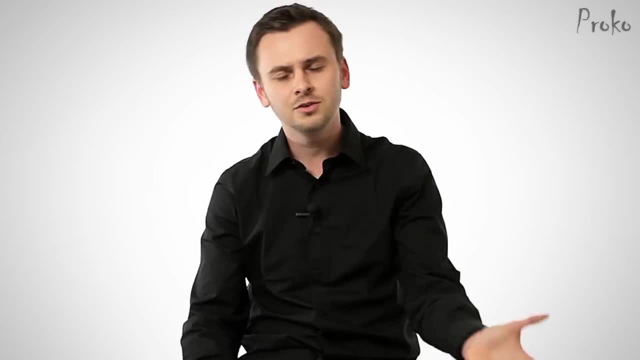 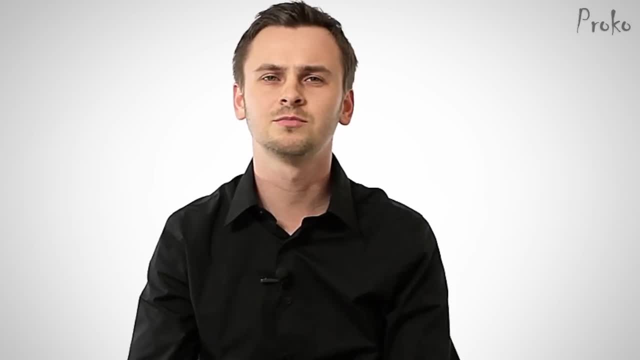 And that's how you get the hang of colors. And that's how you get the hang of colors. But I don't want to make it seem like color isn't important. It is. Colors are beautiful and quite often it's what will catch the eye of somebody looking. 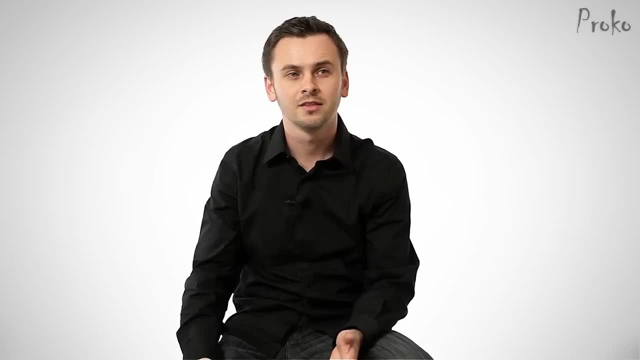 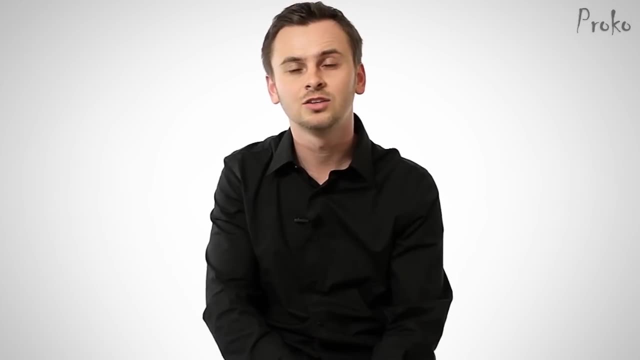 at your artwork. It could set off an emotional response that a grayscale drawing just can't do. But as the artist, you must understand that if you don't get the values right, the rest of the colors won't look right. So focus on accuracy of values and that will allow you to experiment with color and bend. 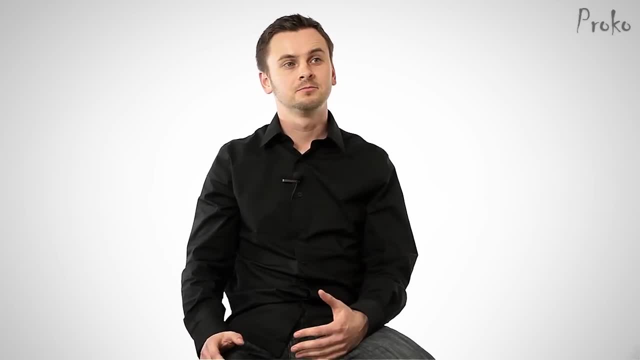 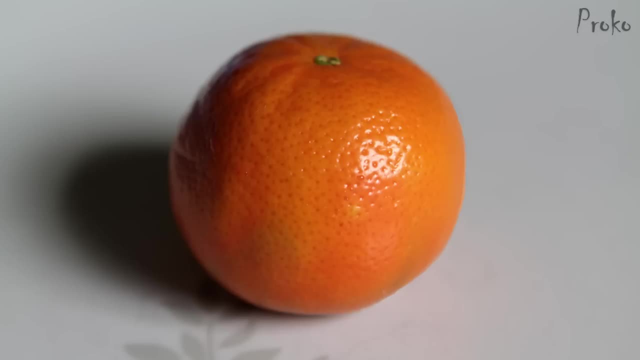 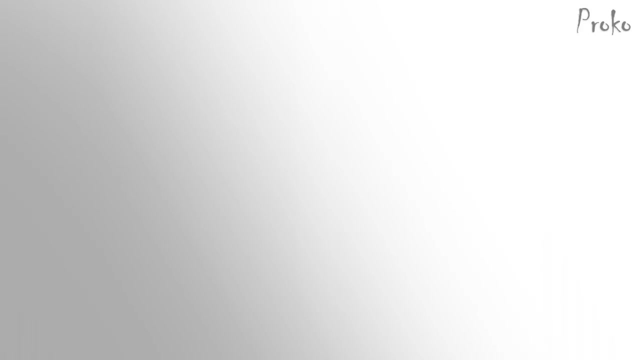 the color. So that's your color basics. Let's move on to edge. Edge is a transition between two shapes. It doesn't have to be the edge of a volume. The shapes within the volume have edges too. The types of edges range from sharp to extremely soft, with an infinite amount in between. 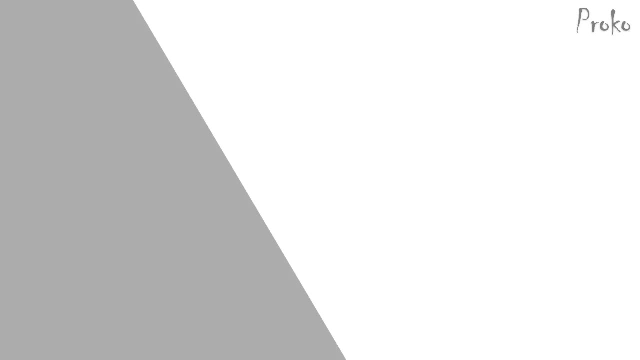 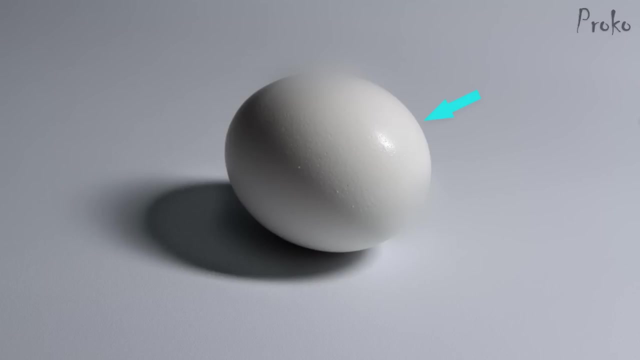 But to simplify it, we've come up with four types of edges: Sharp, Firm, Soft And lost. A sharp edge is a very sudden transition between two shapes. It's sharp like a razor blade. There is no transition, It's a sudden change. 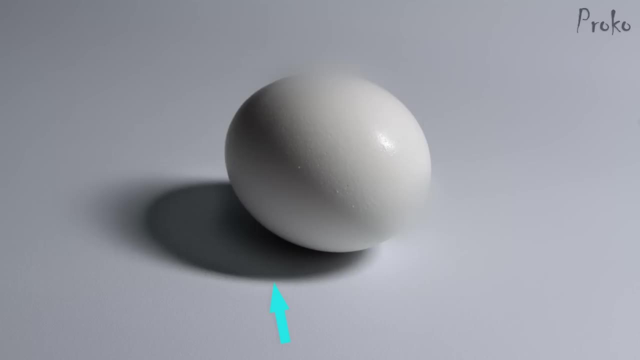 A firm edge is almost hard but has a very small gradation On a figure. you'll typically see firm edges on tendons and joints. A soft edge is a very smooth transition between two shapes. You'll see a longer gradation. 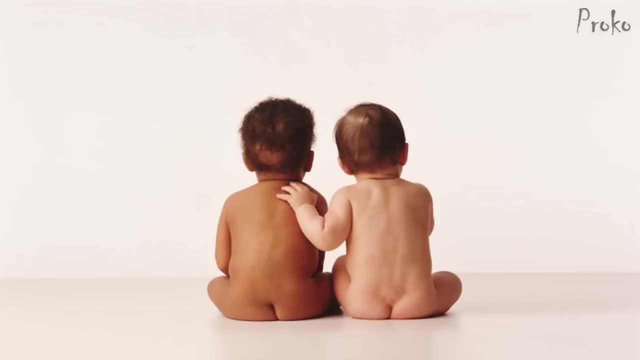 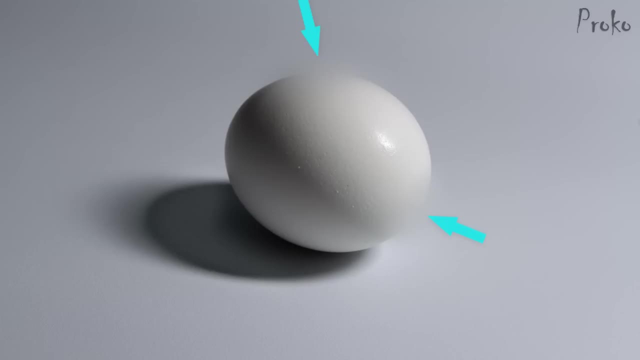 Soft edges are like clouds or baby butts. A lost edge is one that is so soft that you can't see it anymore. It's frequently used in areas where the values of two forms are close together, and a really soft edge would merge the two volumes together. 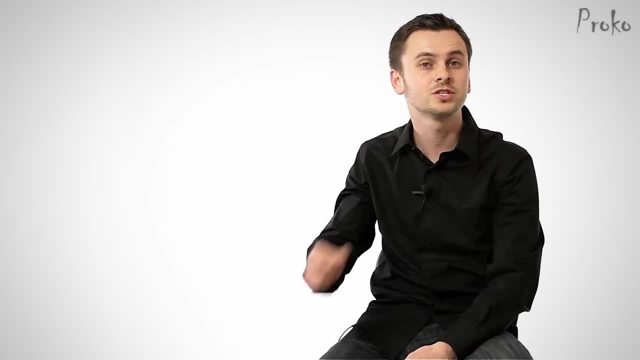 Every time you're drawing or painting, you need to have an intuitive checklist of elements. You just have to plan your drawing and you'll get the results. checklist of elements to identify What is the shape, color and edge And within color. 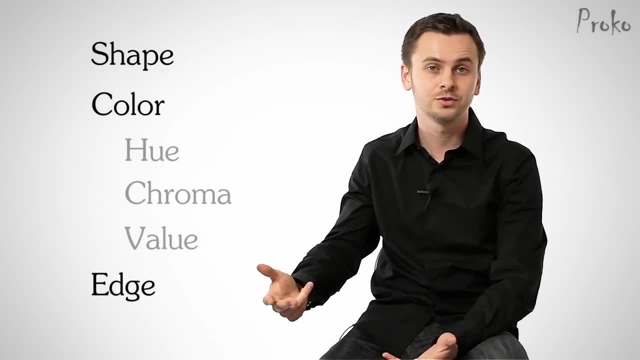 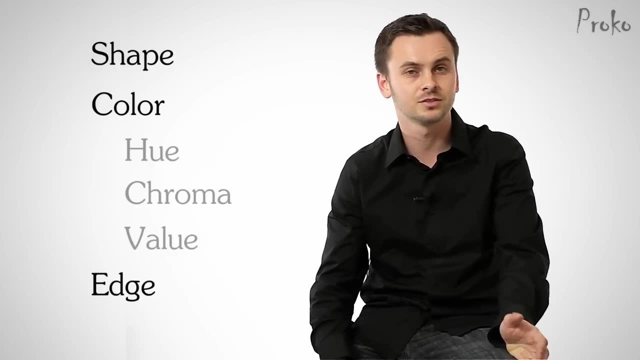 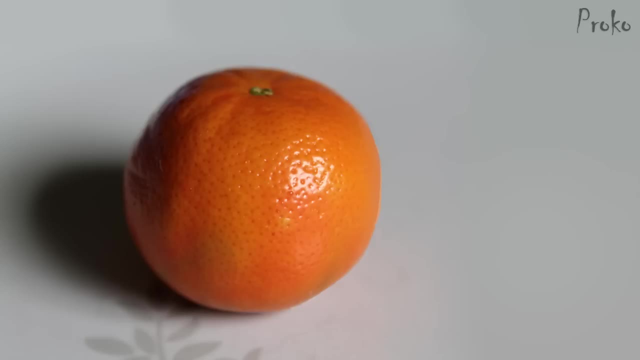 what is the hue, the chroma and the value. To make this intuitive, you have to train your brain to intentionally think about these things as you're analyzing the subject. Eventually, you don't have to force it anymore and it just becomes part of your observation process. 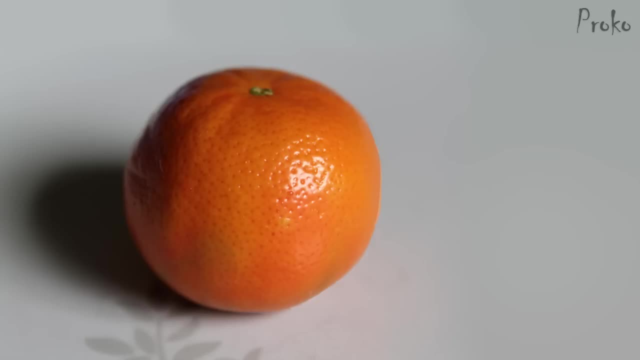 For example, as you look at this clementine and you observe the shadow, ask yourself: what is the shape? Is it circular, rectangular, triangular, etc. In this case, it's a crescent, if you simplify it and something like this. when you look at the details, What is the? 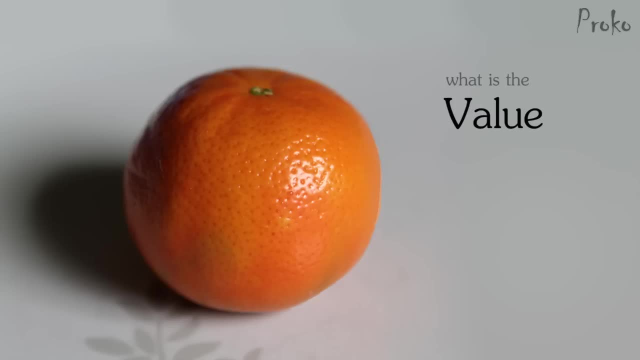 value on a scale of 0 to 10? And, more importantly, what is the value in relationship to all the other values in the picture? This shadow is the darkest part of the picture, So if you want your picture to have the full, 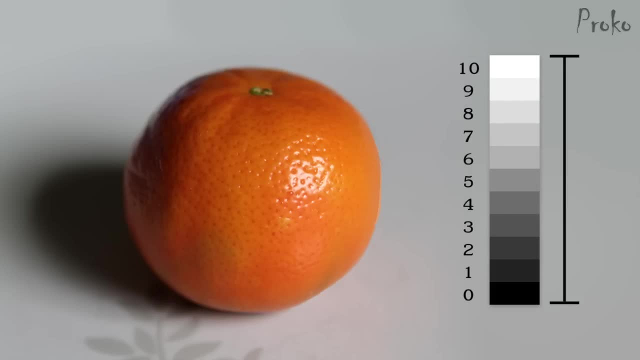 range of values from 0 to 10, you have to make it a value 0.. The top part of the shadow on the clementine is about one value lighter than under the clementine. The reflected light down here is another 1 to 2 values lighter. 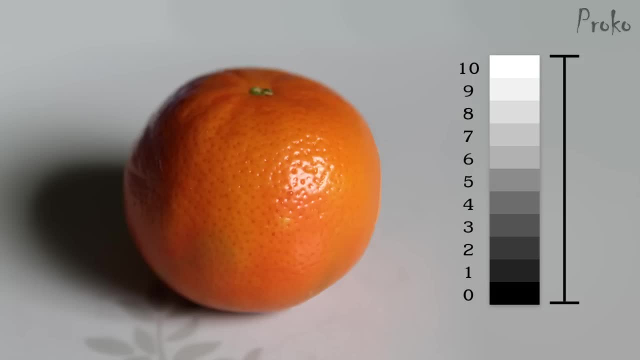 Instead of the full value range from 0 to 10,, you can choose to go for a narrower value range, Let's say 3 to 7.. In that case, this darkest part would be a 3, and the highlight would: 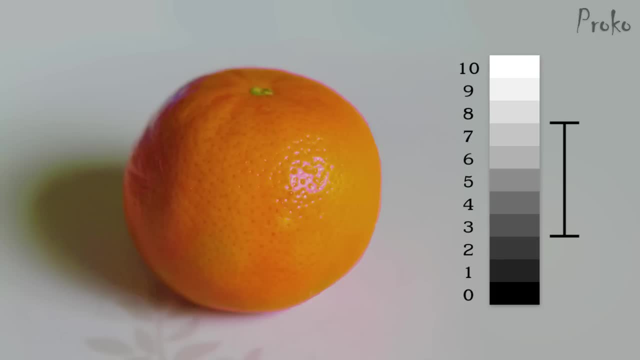 be a 7, and accommodate the other values to fit within that range. So it's the relationships between all the values in the picture that really matter. The next question is: what is the hue? Even though it's an orange clementine, not all. 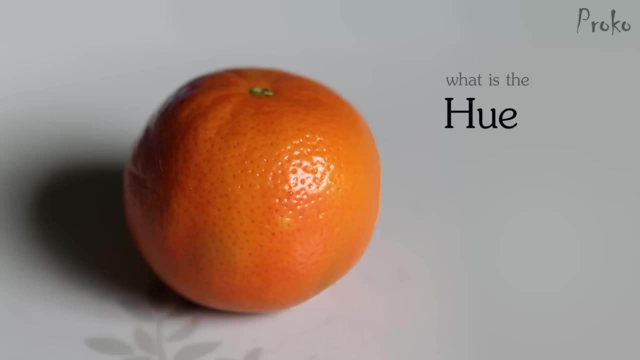 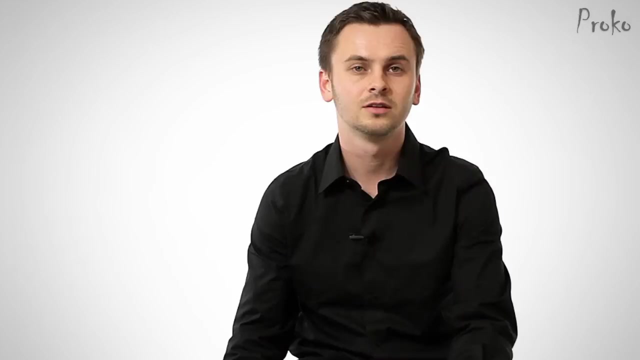 the colors on it are orange. I'm seeing a transition from orange on the light side to a redder hue on the shadow side. What is the chroma? It's somewhere in the middle, probably a little closer to the high chroma side, And the edge is firm on the left side and softer on the right. 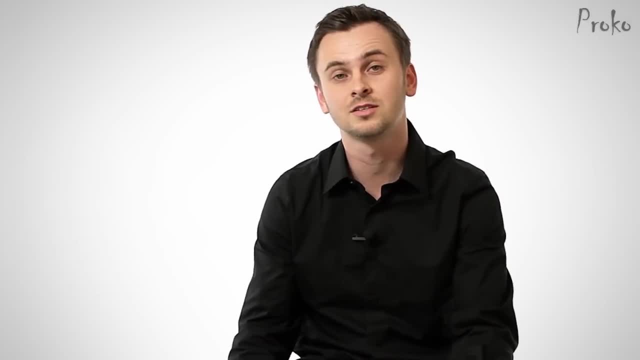 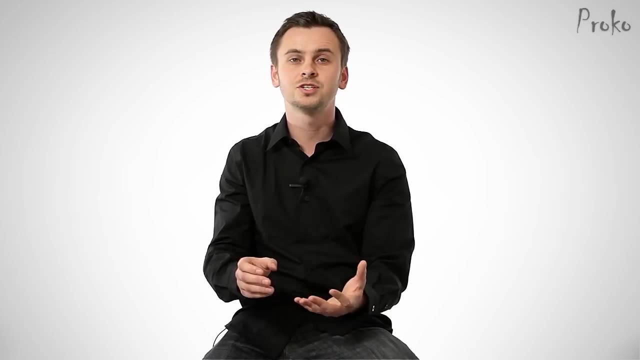 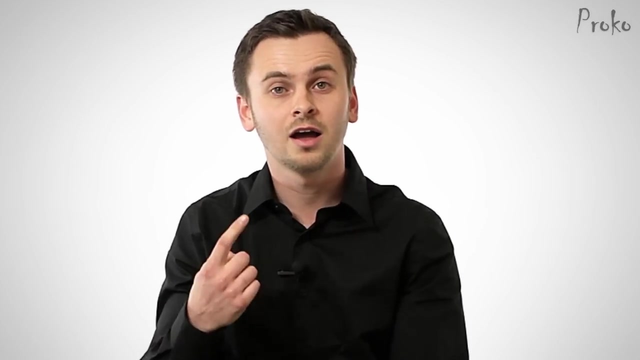 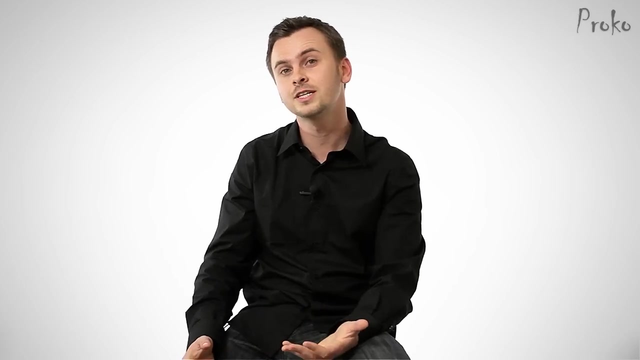 The ability to see and properly identify these elements is a skill. It's a sense that you need to develop. At first you will struggle to see these subtleties, But, just as a musician, you will be able to see the world through an artist's eye. As with most things, it's. 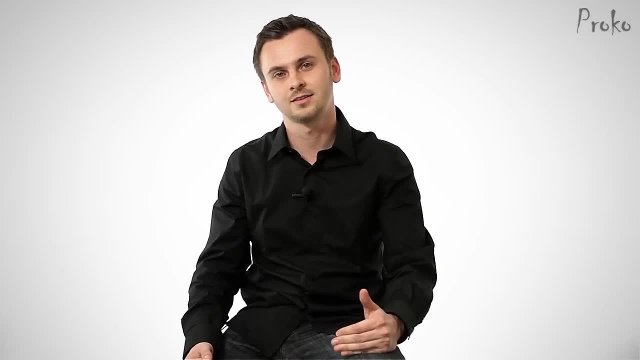 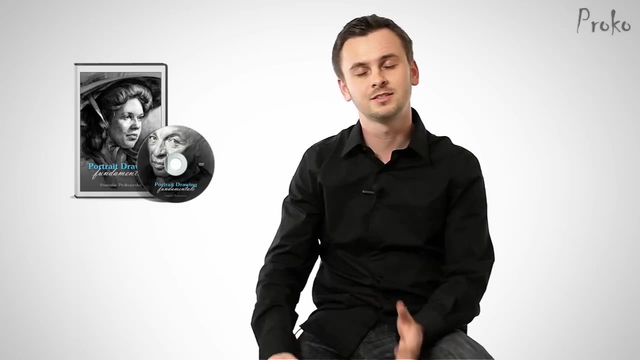 about repetition- repetition through practice. Before you go, I want to thank everybody who bought my portrait drawing DVD. You guys have been really, really supportive and I owe you a big thank you. If you don't have one yet and want to learn more, check out the link in the description below. 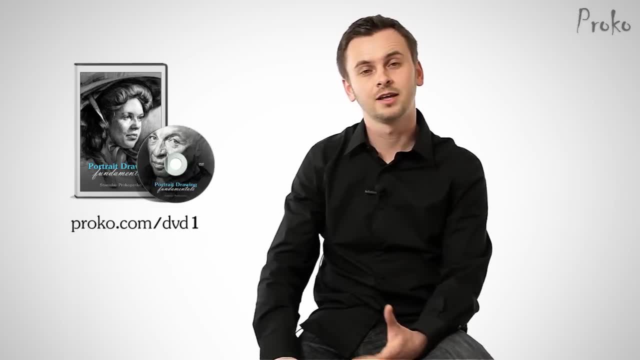 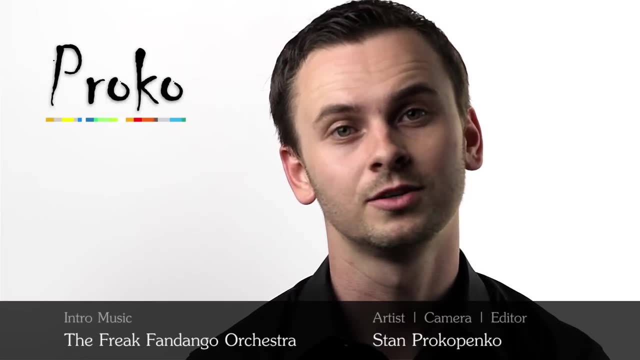 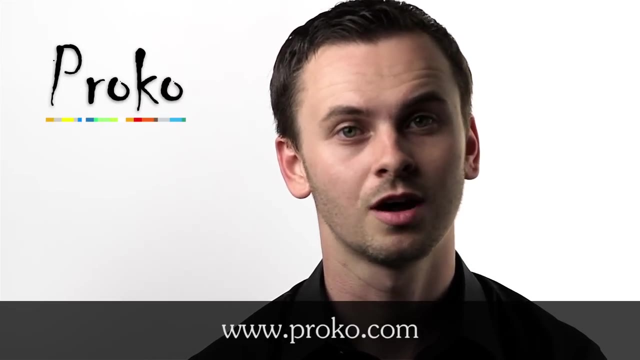 Hey, if you liked this video, your friends might too. Please help me out and share this video on your favorite social network, And don't forget to subscribe to the newsletter on prokocom.